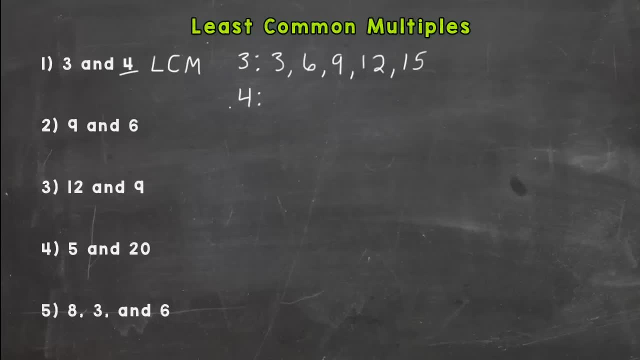 four can multiply into, And the easy way to write out the list is just count up by four. Four, Eight, Twelve, Sixteen, Twenty. All right, so there are our multiples lists. We need to see if they have any in common, any they share any partners here. So you look at both, both lists, and it looks like. 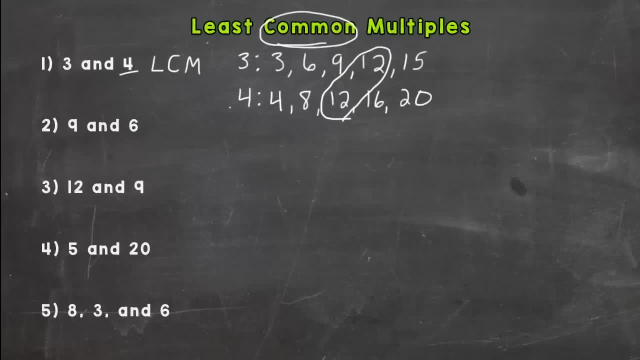 they have a twelve, forty And there's an in common and there aren't any more that they have in common. If we were to continue these lists on, we would find more they have in common, but we don't need to find more they. 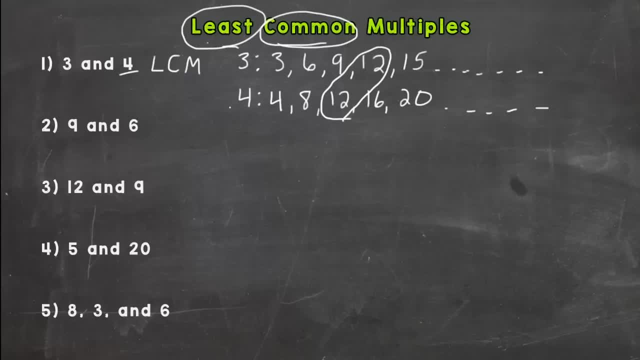 have in common. We want the least they have in common, and there aren't any less than twelve. so our LCM, or least common multiple for three and four, is twelve. That's our answer. Now, if we were in our fraction unit, we would use that 12 and apply it to a certain type of problem. So we would use that. 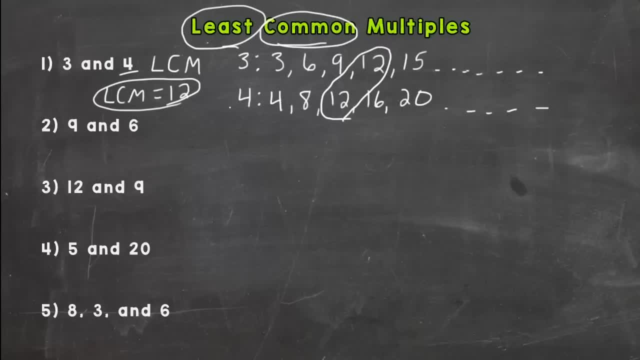 12.. So it's very, very important we know how to find the least common multiples. So let's go to 9 and 6.. We'll make our multiples list for 9 and 6.. So 9,, 18,, 27,, 36.. 6,, 12,, 18,, 24.. Do we have any? 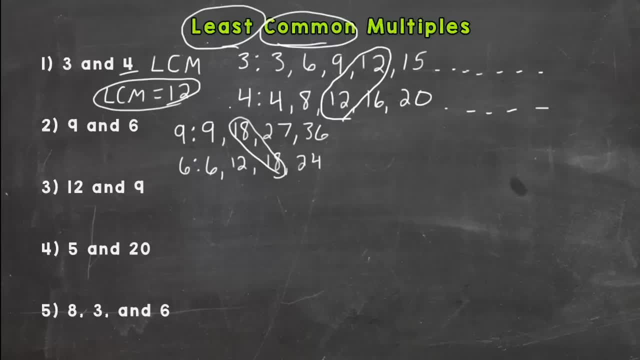 in common? Yes, the 18.. Let's see if we have any less than that. It doesn't look like it. So our LC For 9 and 6 is 18.. If let's say, we wrote out our list for 9 and 6 and we didn't find any, 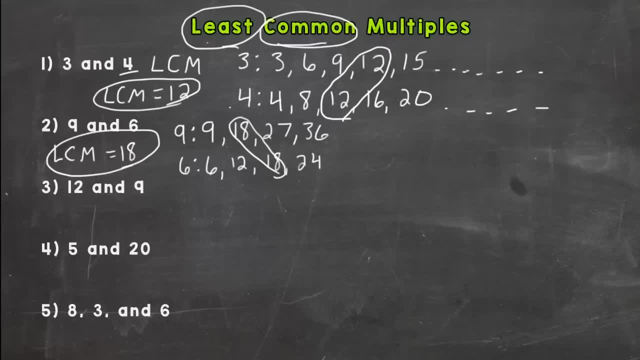 just continue your list until you do find a match. So if you don't see one after you write out five multiples for each, that's okay, It will happen. You just need to continue your list until you find a matching pair. So number three: we have a 12.. 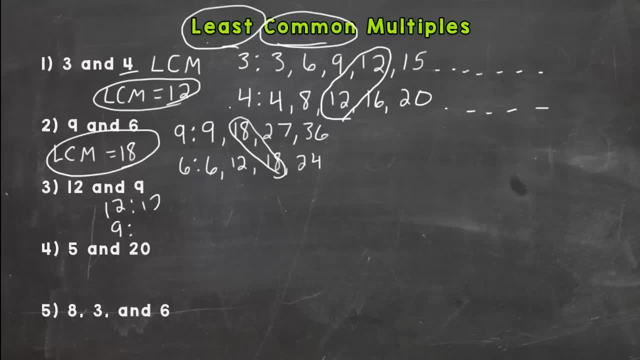 And a 9.. So 12,, 24,, 36,, 48., 9,, 18,, 27,, 36.. And it looks like we have a match there for 36.. Any more Less than that? No, it doesn't look like it. So our LCM for 12 and 9 is 36.. 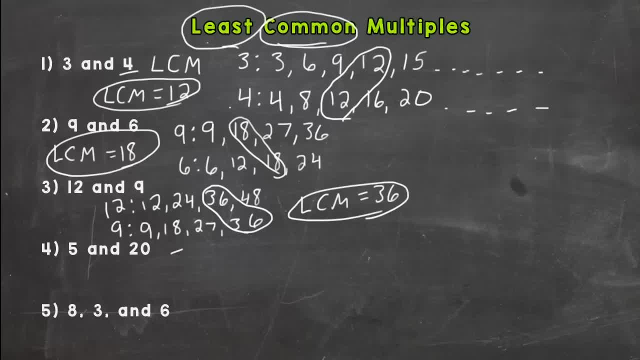 Number four: 5 and 20.. If you want, if you think you have this down, go a little bit ahead of me here for the 5 and 20 and then check your answer with mine. So 5 and 20,, 5, 10,, 15,, 20.. Notice my. 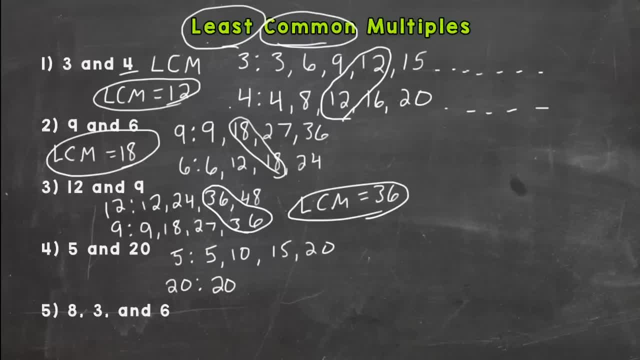 list for 20.. I start with 20. And if you notice that we have a match already, we have a match for 30. There's no need for you to continue your list and go 20,, 40,, 60,, 80. If you notice a match, 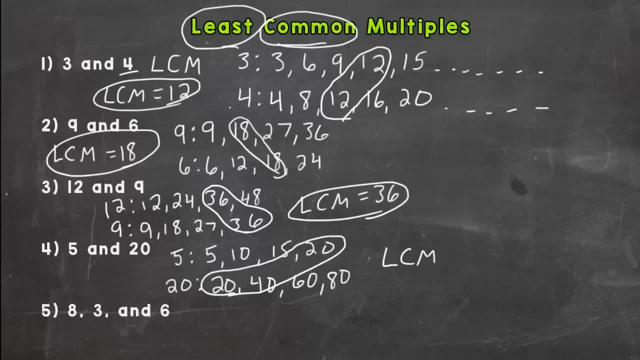 you can stop there. So our LCM for 5 and 20 is 20.. Your least common multiple can be one of the numbers in your problem. See how it matched our 20 there. That's okay, That happens. And then number. 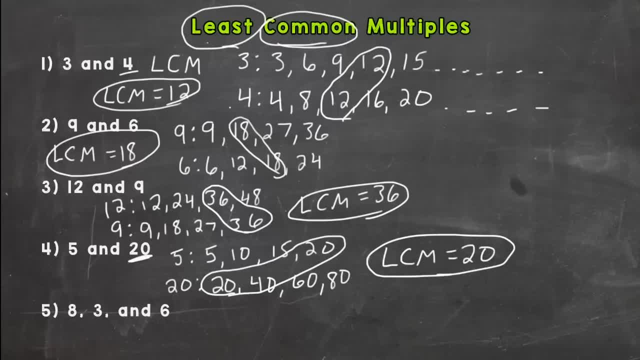 three is the least common multiple between. So you make three lists and you have to find one that all three have in common and the least that they have in common. So I'm going to come over here where I have a little bit more room: 8,, 3, and 6.. So let's start with 8.. 8,, 16,, 24,, 32.. Let's do 3 now. 3,, 6,. 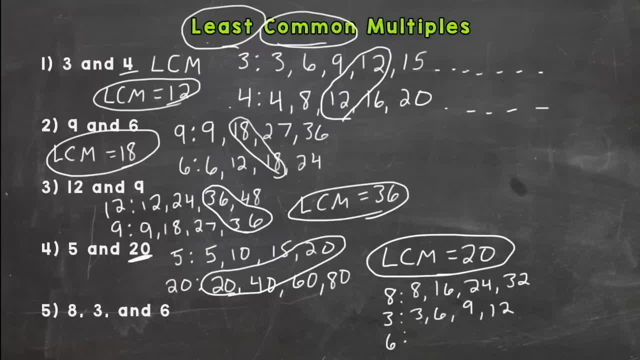 9, 12.. And 6,, 6,, 12,, 18,, 24.. Let's see if we have any in common, And it does not look like we do yet, So we're going to need to extend And notice. my 8 is up at 32 already And my list for 3 is: